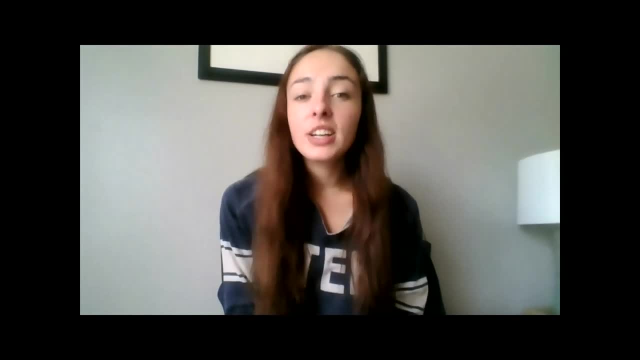 Hi y'all. So today we're going to be discussing geologic time and relative dating. If you don't know what relative dating is, we're going to get into it. Basically, there are two main ways to determine the age of rocks. We use either relative or absolute dating methods, and we'll talk about 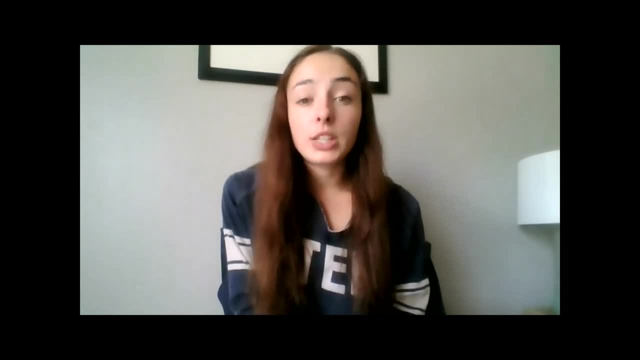 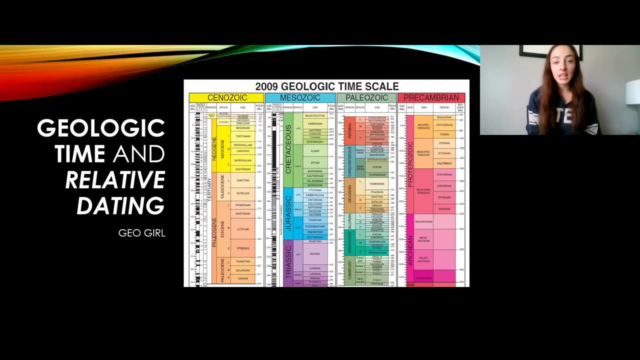 absolute dating next time. So this time we'll discuss both geologic time and relative dating techniques. So let's get started. You can see here a picture of the time scale. This is the geologic time scale, guys. This is the Geologic Society of America or GSA version, but there are 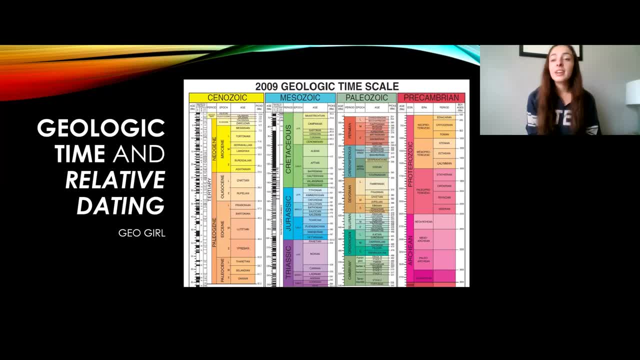 many versions. I like this one because it's colorful. So how you can read this. I know it looks like a lot right now, but basically this is all of Earth's history based on our rock record, meaning we've gone and looked at rocks that are aged throughout Earth's history, from 4.5 billion. 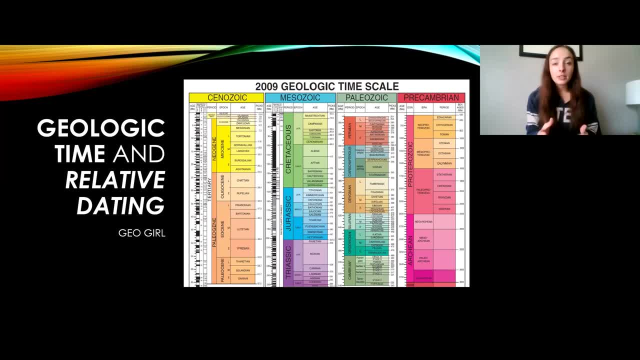 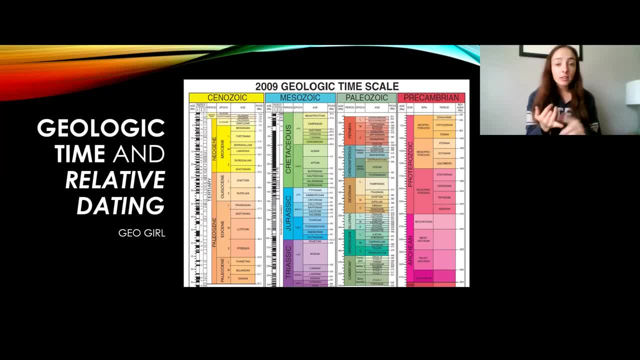 the geologic time scale, guys. This is the geologic time scale, guys. This is the geologic time scale distinguished from each other by different characteristics, like lithology, fossils, and we'll talk about what that means. But basically that's how we came up with the. 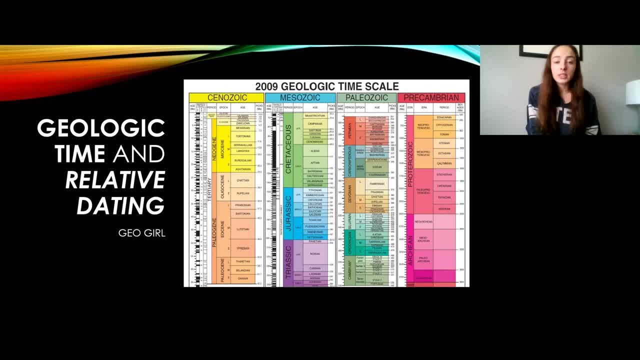 different categories And in this time scale you can see that the age is shown in the very left column of each main column. That left column says age and then it says ma. Ma just means millions of years, So that's a unit of age And so all these numbers are in millions of years. You 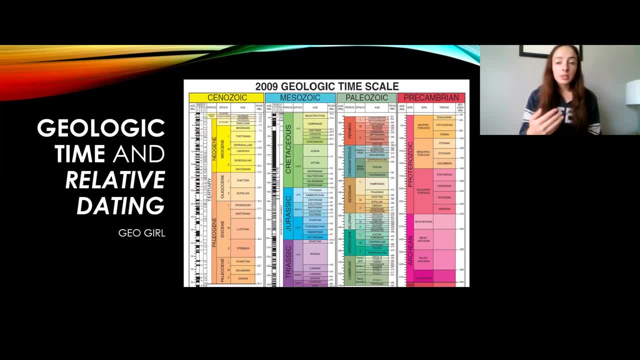 see like 25,, 25 millions years ago. So that's the age in millions of years, And so you can see the time scale goes all the way back. Well, you can't see the very bottom because it cut off in the picture, but it goes back to 4.5 billion years ago, at the beginning of the Hadean, I mean. 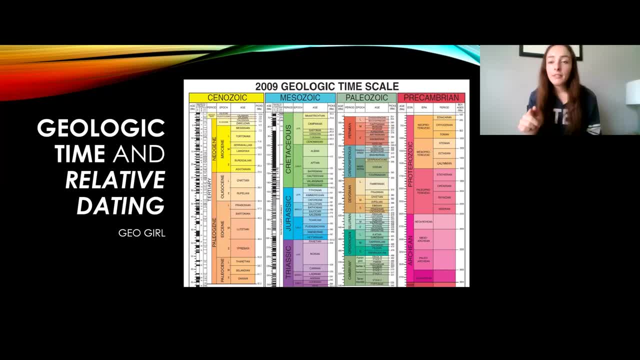 that is all the way on the bottom right of that figure. So it starts at the bottom right and goes up from the Hadean to the Arkan, to the Proterozoic, and it goes back down. You see that where it says: 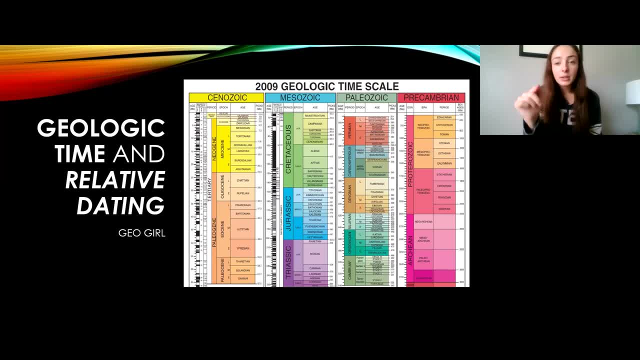 Cambrian, if you go one more column to the left and then it goes up to Permian, and then it goes back down to Triassic, and then up to Cretaceous, and then back down to Paleogene, and then up to Neogene, And that is how you can read this time scale And basically each main. 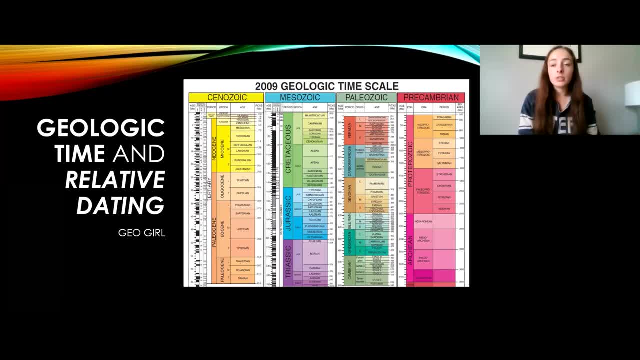 column, those color-coded columns, one with the headings. those are the Precambrian, then the Paleozoic, then the Mesozoic and the Cenozoic. And the Precambrian is broken up into three different eons. An eon is the largest time unit that we'll see. It's kind of weird, though. 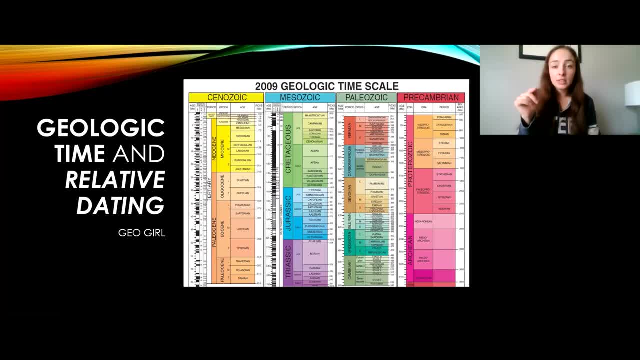 because the Precambrian designates all three of those eons. but it's also an eon, Don't think about it too long. The Precambrian consists of eons- Hadean, Archean and Protozoic. Then you can break that down into eras. Then you can break 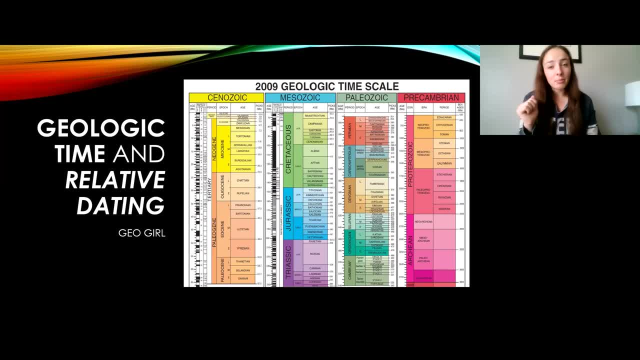 those down into periods, And that's so long in time ago that you can't really break the periods down into epochs and ages, like we'll see in the rest of the eras. But you get the gist. Then from the Precambrian we go into the Paleozoic, Mesozoic and Cenozoic And all of 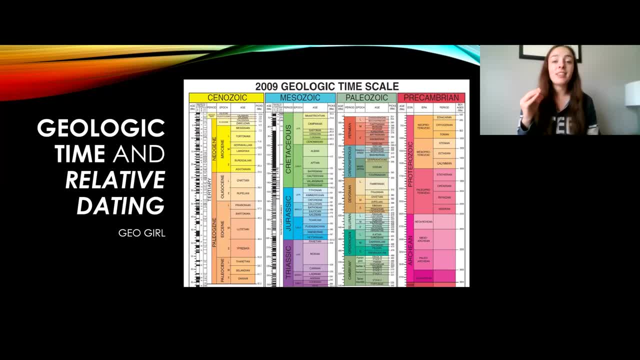 those eras. those are eras are designated within the Phanerozoic eon, So it's Precambrian, which is composed of Hadean, Archean and Protozoic eons, And then from those it goes to. 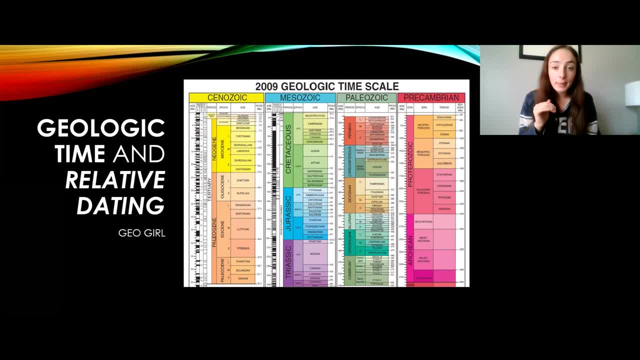 Phanerozoic eon. That eon is composed of the Paleozoic, Mesozoic and Cenozoic eras, So eon, era period and then epoch and age. The Paleozoic is broken up into the Cambrian Ordovician. 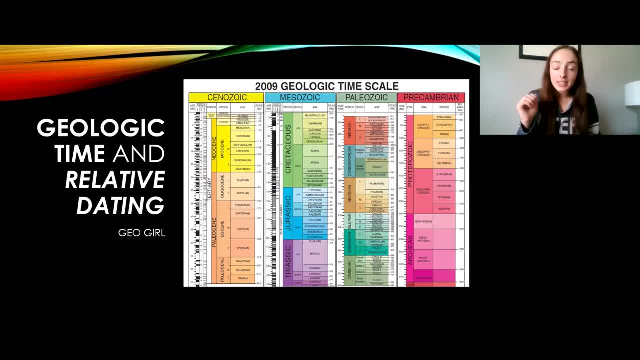 Silurian, Devonian, Carboniferous and Permian periods. These periods can be further broken down into epochs or epochs, whatever you want to pronounce it, And then those epochs can be broken down into ages, And those are typically only used by the people that are studying a very 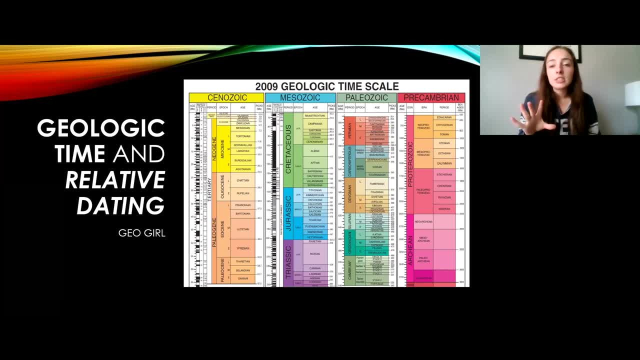 specific time in our society. So don't worry about the ages or even the epochs. Focus on periods are really important, And then, obviously, eras and eons. Moving on to the Mesozoic, you can see that we have the Triassic, Jurassic and Cretaceous periods. Those can be broken down further into epochs. 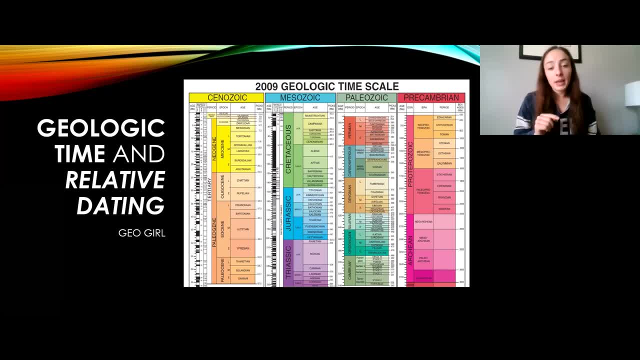 and ages. And then, moving on to the Cenozoic, we have the Paleogene and Neogene periods, But in the Cenozoic we typically use epochs because so much more is known about more recent rocks, because we have so much more rocks in recent time than we have in the past. So we 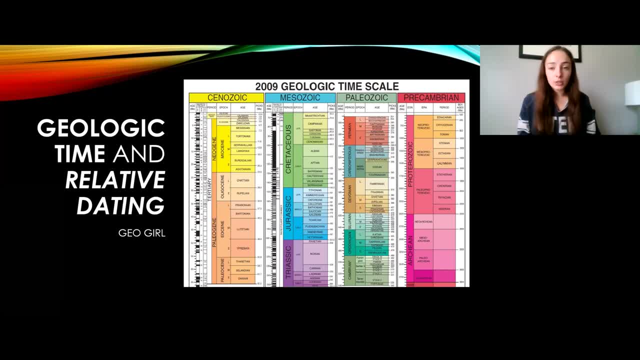 have from the Precambrian because those have been recycled or destroyed by erosion or whatever it might be. So we have way more in the Cenozoic rock record than we do the others. So we use epochs because we can get more specific. there We have more information. So with the epochs of the 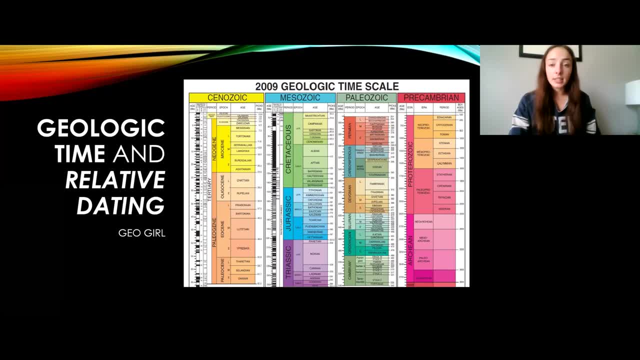 Cenozoic. we have the Paleocene, Eocene and Oligocene for the Paleogene period, And then the epochs for the Neogene period are the Miocene and Flyocene. Then the last period is the Quaternary. 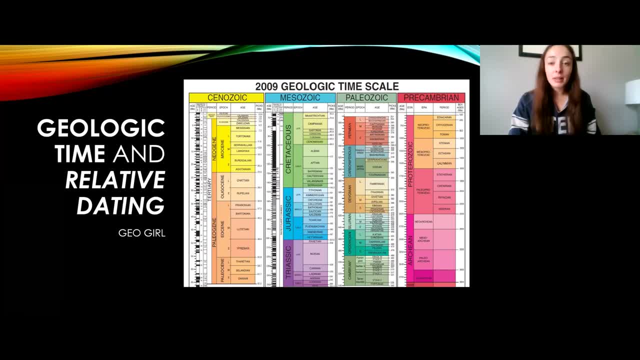 and that's what we are in right now. And you can break that up into the Pleistocene and Holocene epochs. And now some people are saying that we're in a new epoch, that is the Anthropocene, but I don't know how scientific that is, So we're in the Holocene. We'll just stick with that. 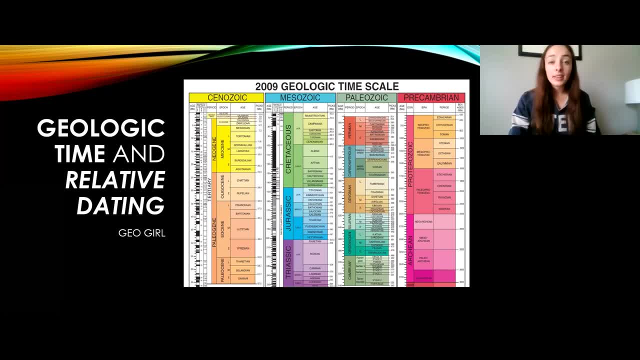 Anyway, that's how you can break down the categories of the timescale with my later episodes that are going to be over- exactly what happened or what evolved on Earth in the specific eons and eras and periods of Earth's history. A lot more used to hearing these time categories stated in sentences and kind of understand what. 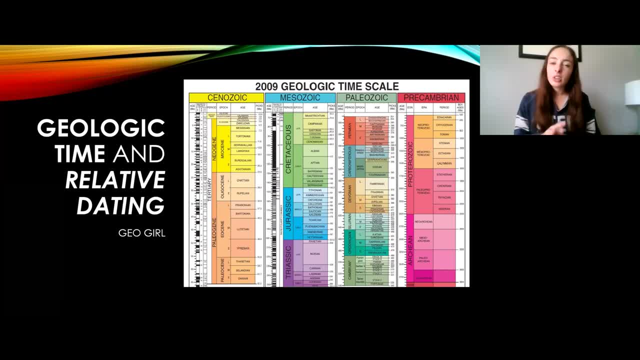 happened during them, And that way you'll remember it more. But for now that's all you really need to know how to designate each time category and what they mean, And that's enough for now. So let's move on to how to think about geologic time. In this slide we can tell: 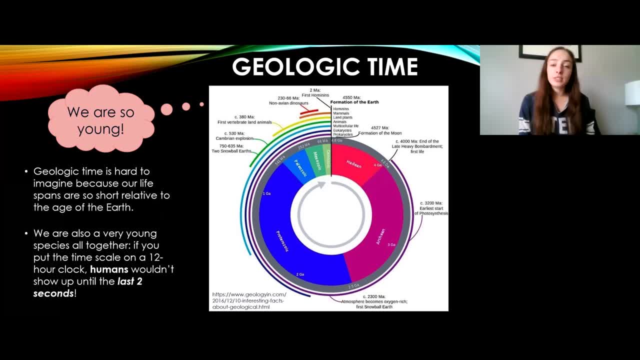 holy crap. we're a young species. So, for example, this is a circular geologic timescale. This shows how long major things have been around. For example, photosynthesis started over 3 billion years ago And you can see that on the right side in the Archean Eon And if you go forward. 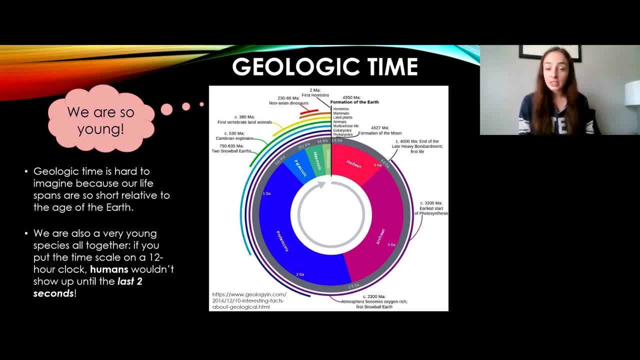 you can see when the Great Oxidation Event occurred. We're going to be talking about this for a whole episode. It's so important and awesome. But the Great Oxidation Event- basically it says here at the bottom- when the atmosphere became oxygen rich. 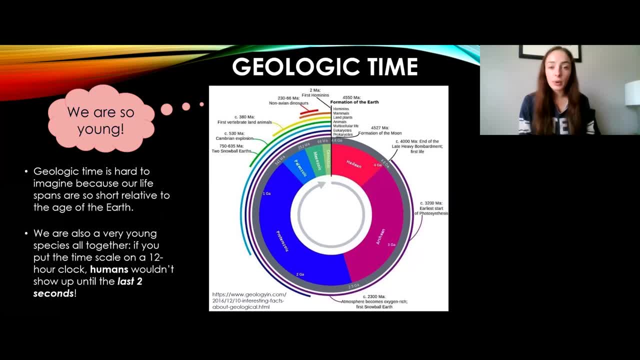 that's a really important time And that was around 2.4 to 2.1 billion years ago And that's in the Proterozoic Eon, And then moving forward, you can see when dinosaurs came around and then died out in the 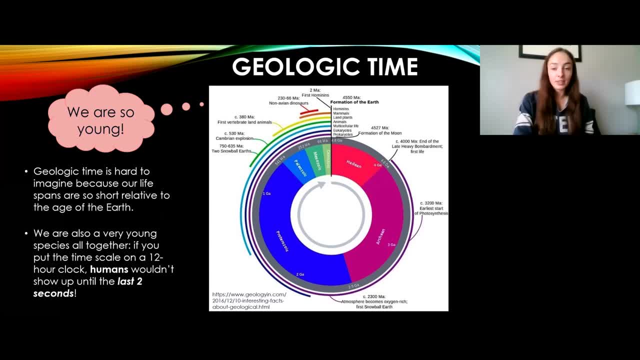 Mesozoic, almost at the very end of the timescale compared to the rest of the time, And then you can see. well, let me take that back. You can't see really well where the first hominins came in, And 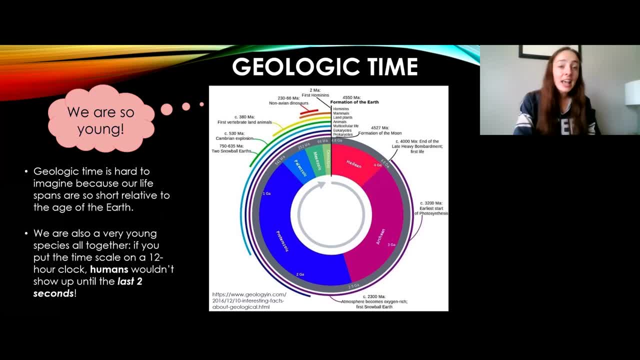 that's the lineage that we came from. So it's kind of crazy how young of a species- and not only species but family- we are, And we'll talk about the different categories of taxonomy and later episodes. But my goodness, we are young, And I emphasize this by another cool fact. 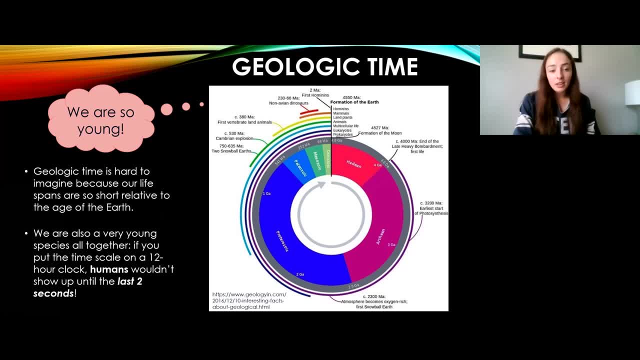 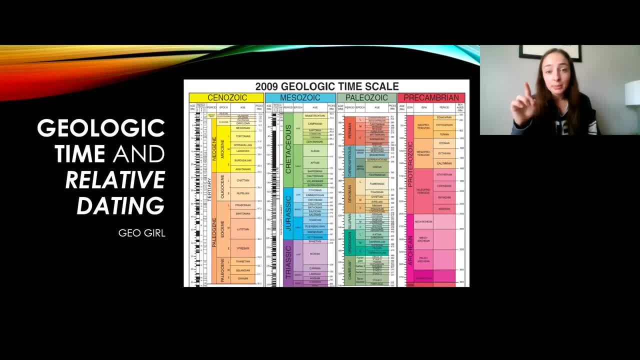 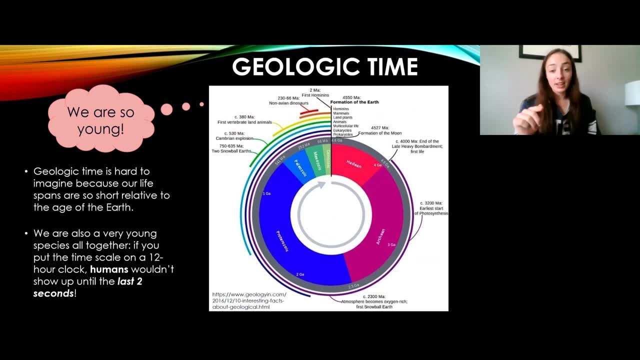 that first column. on the last picture, if you go here, that's just the Precambrian. That consists of the majority of Earth's history. You can see that with this circle graph. That's why I like the circle graph, but it's also like mind-blowing. Most of Earth's history was just magma at the 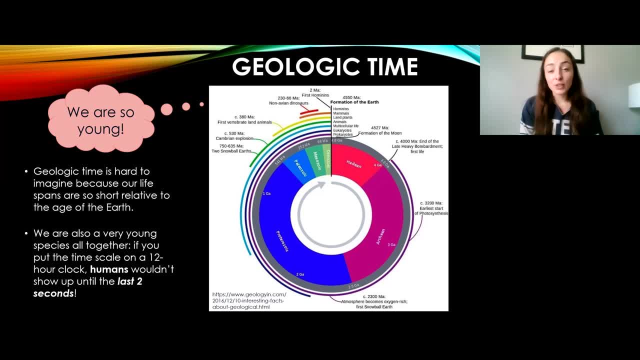 beginning, then an ocean, then life. This life was not what most of us think as life. It was just single cellular organisms, microbes and whatnot. for a long time, Even the photosynthesis microbes, They were not plants yet. They were plants way later. We all are very young. 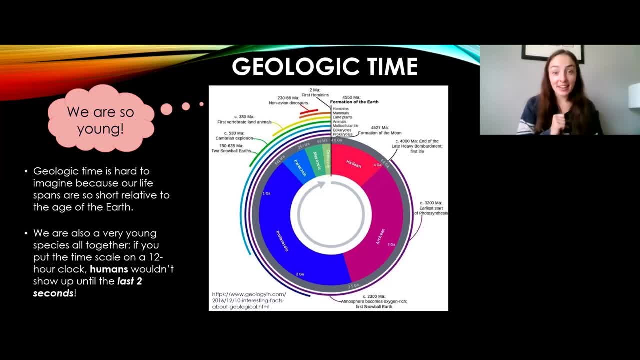 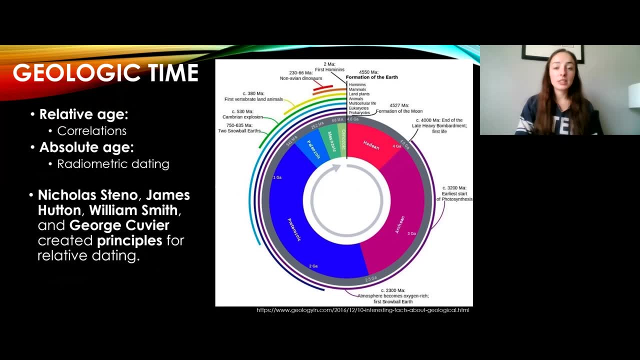 even the dinosaurs. They're still here as birds and they're still young compared to the rest of Earth's history. Now getting into the difference between relative and absolute age. Relative age is how we determine a rock's age, using relative dating or relative techniques, meaning relative. 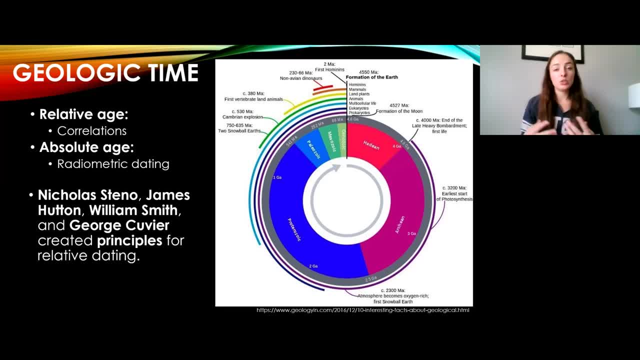 to this rock. this rock is older A lot of times. that's easy because you can walk up to an outcrop where there's a few layers and you could say, well, that layer on the bottom should be the older than the layer on the top, because you know gravity. But actually we have a principle. 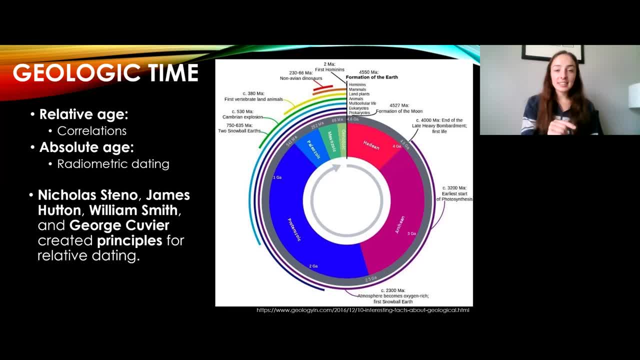 for this, and we're going to go over principles of relative dating in the next slide, And the people that made these wonderful principles that are very useful for relative dating in geology are Nicholas Steno, James Hutton, William Smith and George Cuvier, And these are going to be the. 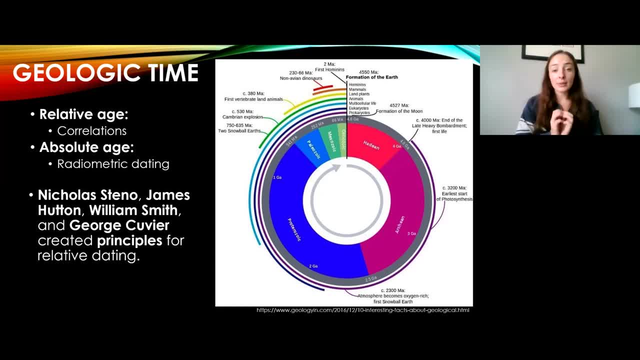 principles of relative dating that set the stage for allowing us to date rocks, because relative dating came along way before absolute dating, which we'll talk about in the next episode. But, as you can see, we're going to be talking about relative dating in the next episode. 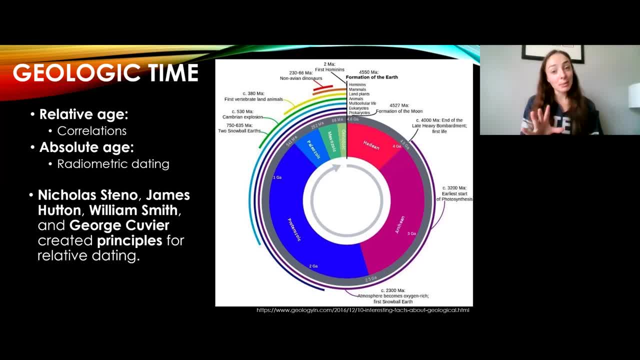 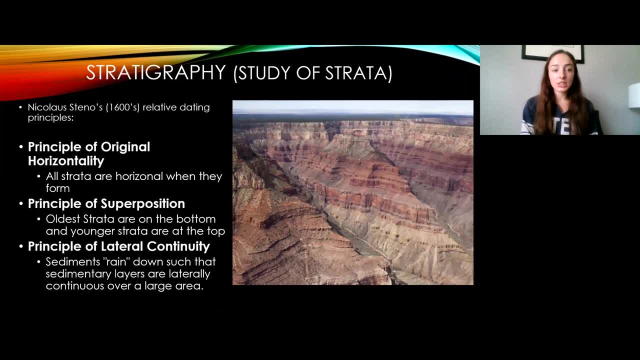 As you can see here, it involves radiometric dating, So it sounds a little bit more quantitative, which it is, but relative dating is how we made the geologic timescale, So let's see how it works. The principles include the principle of original horizontality, which just means that all strata 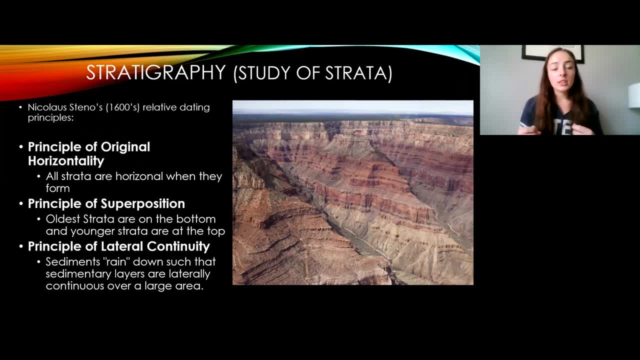 were horizontal when they formed. Strata are just layers of rocks, And so if you come up to an outcrop where there's layers that are not horizontal- they're layered, but they're tilted or folded or something- then that means that that tilting and folding must have happened after. 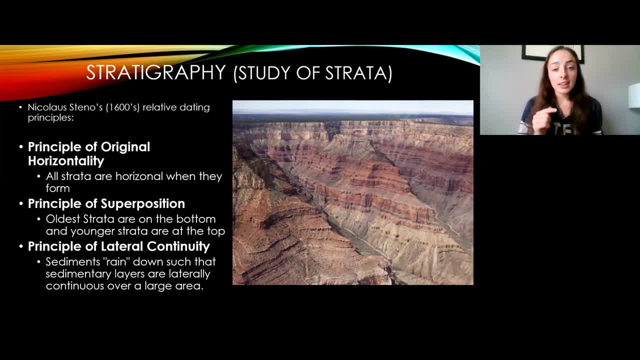 they were deposited Superposition. this principle states, like I said earlier, if you see layers of a rock, the older one is the one on the bottom, the younger one is the one on the top, And this seems very simple, but someone did have to come along and say it and actually put it in writing And 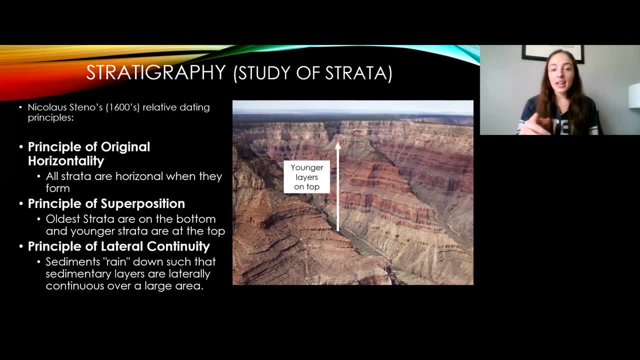 now we can use it. And that person was Nicholas Steno in the 1600s And you can see this principle here, in these strata- in the picture to the right you can see the younger ones are on the top- And then principle of lateral continuity, which you can also see in this picture, is basically saying 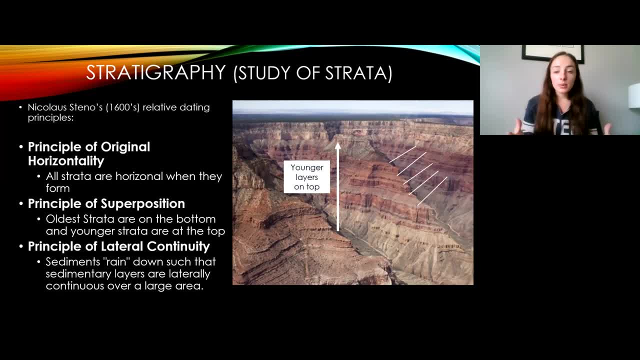 sediment rains down or gets deposited in a way that is laterally continuous. So you know, if you have this canyon type erosion, where you have these layers in this one pillar of rock and then a pillar over there, but you can't see the in between, you can infer that there was rock in. 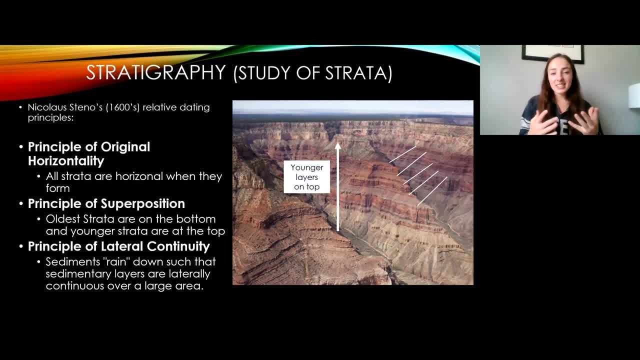 between if those layers look the same and like they match up. it's typically pretty self explanatory as well, But again had to come along and say it. And these are three principles that Steno has blessed us with And we can use them to explain the structure of the rock, And we can use them to 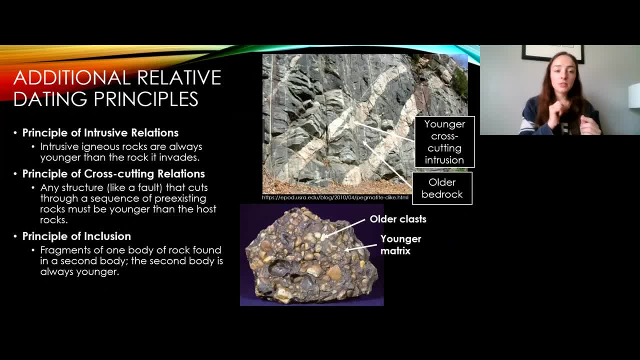 relatively date rocks. Additionally, the principle of intrusive relationships states that igneous rocks that intrude original sediment are younger than those original rocks, And we can tell things like this because typically those intrusions are cross cutting layers And that goes into the 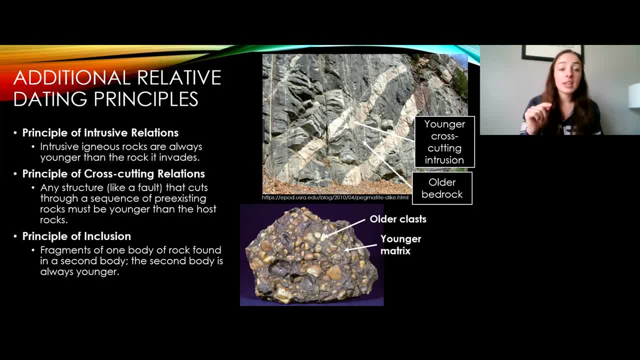 principle of cross cutting. principle of cross cutting relations states that a structure, such as a fault that cuts across layers, is also younger than those original sediments. So the intrusive cross cutting relations I find really similar. They're basically if an intrusion is cross cutting. 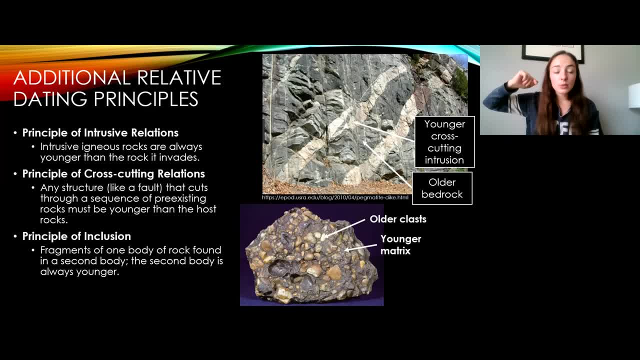 or a false cross cutting the original strata- and you can see that with your eyes- then you know that that intrusion or fault or whatever is younger And so they're very similar. cross cutting just typically refers to faults. Intrusive relations just typically refers to igneous. 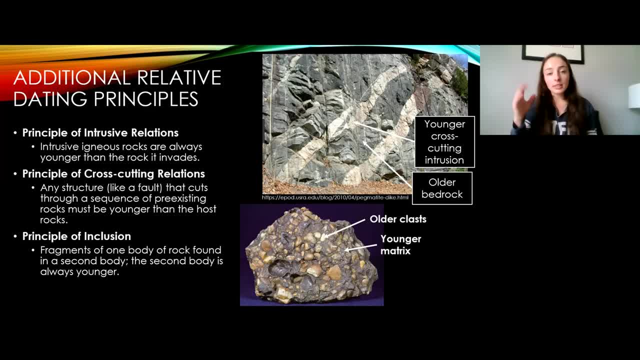 intrusion, because magma is the only thing that causes, like dikes and sills, to come up and intrude original sediment. So the last one on this slide: the principle of inclusion states that fragments from one body of rock found in a second body are older than that second body. 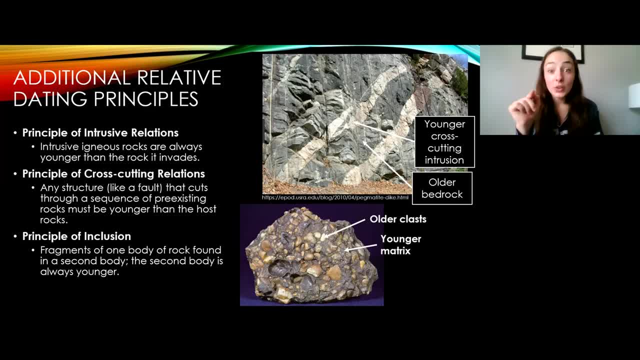 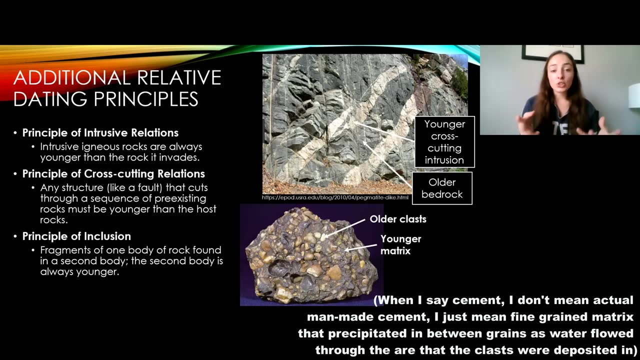 meaning, if you look at this rock that has all the class that we know is conglomerate from previous episodes, that these class are from sediment that was eroded and watered from something else that then got re cemented together into a new rock and the cement part is the matrix and these class are. 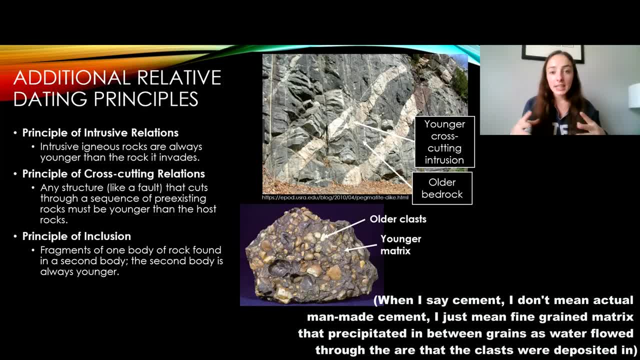 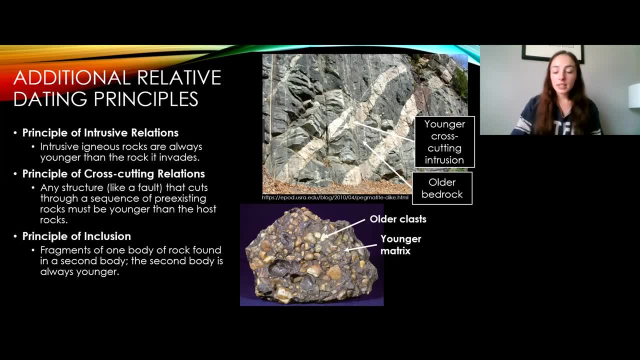 older than the matrix because they were around and then they got cemented together by new or younger cement. So that is the principle of inclusion. And then the last one on this slide. the principle of inclusion is the relative date between those class and the younger matrix. That is it for relative. 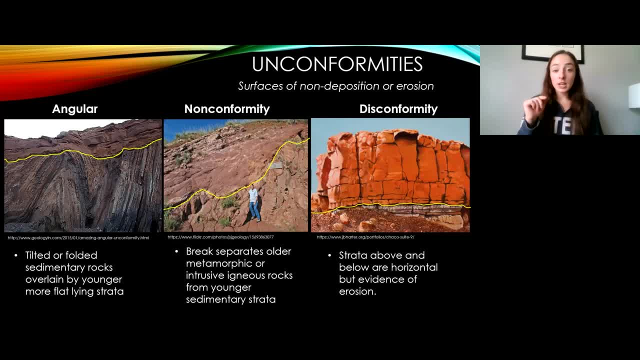 dating principles. There are more important concepts to know, For example, unconformities. These are really important for relative dating because unconformities represent surfaces of non-deposition or erosion. These are important because you can't just go and say this stratum. 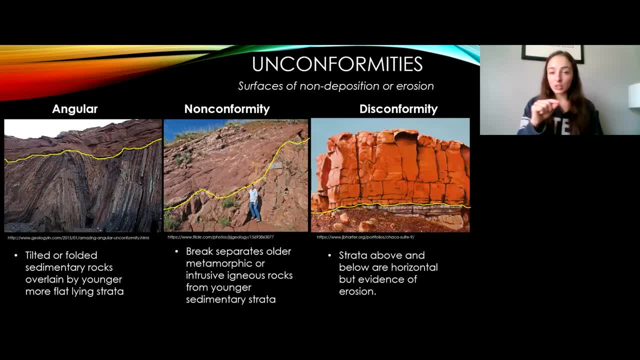 was deposited, and then this one was because maybe there's an erosional surface there. there was time in between there. that could be short, it could be super long, it could be millions, billions of years. We don't know until we do some. 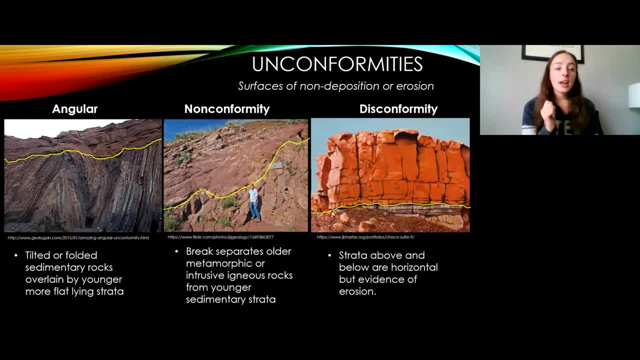 further investigation, which is what unconformities call for. And we can recognize unconformities by looking at the surfaces between rock layers or boundaries, And three main types of unconformities include angular unconformities, nonconformities and disconformities. Angular unconformities are: 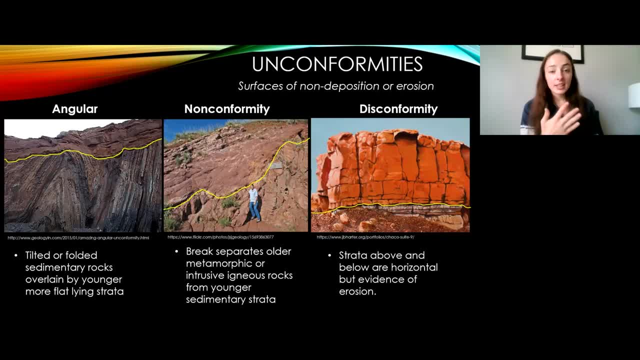 probably the easiest to recognize. You can see here on the left. basically, if layers are angled or they were folded somehow and then erosion occurred, cuts on a straight line over that angular surface and then more sediment was deposited. on that you can tell there was. 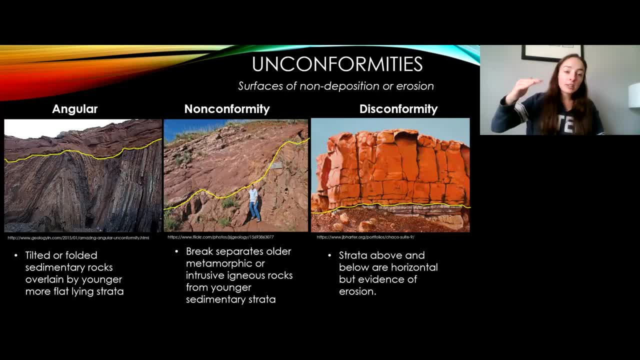 erosion and missing time, because clearly where the layers are angled you can't see the top of that fold. so something was cut off A bunch of time. there was just cut right off and then more layers were deposited. so you have a lot of missing time there. That is the easiest to 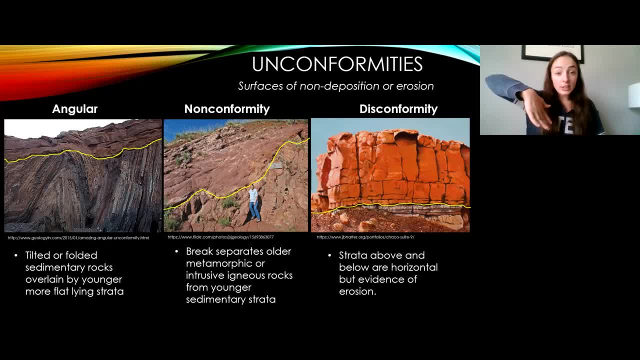 recognize because the angular unconformity has angular layers right underneath it and cuts them off. So that's an angular unconformity Moving on to a nonconformity. Nonconformities separate metamorphic or igneous rock from younger sedimentary rock, If sedimentary rocks are. 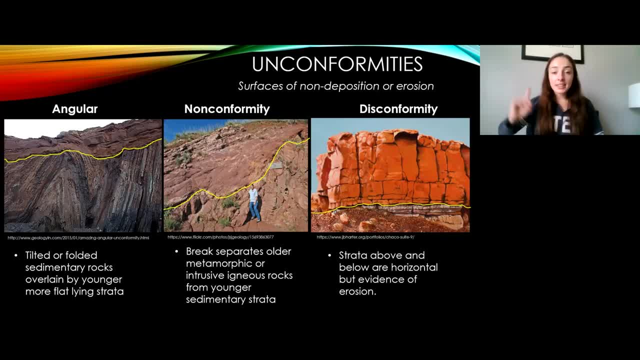 deposited right on top of some metamorphic or igneous rocks. that's a nonconformity And you can tell there's missing time there, because sedimentary rocks aren't necessarily being deposited or formed where igneous and metamorphic rocks are formed clearly. So we know there's. 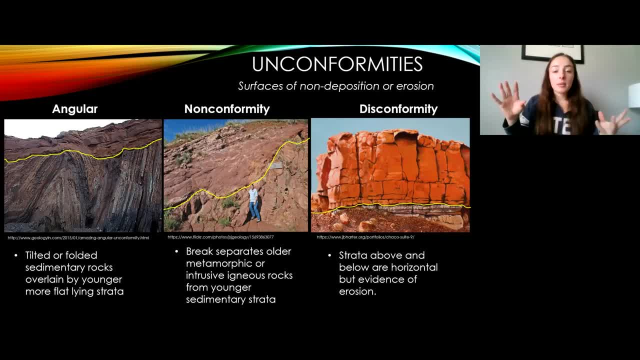 missing time there and igneous and metamorphic rocks were there, and then a bunch of erosion occurred- uplift and erosion or whatever it might have been- and then sedimentary layers got deposited on top way later, And then the disconformity might be the most inconspicuous one, meaning 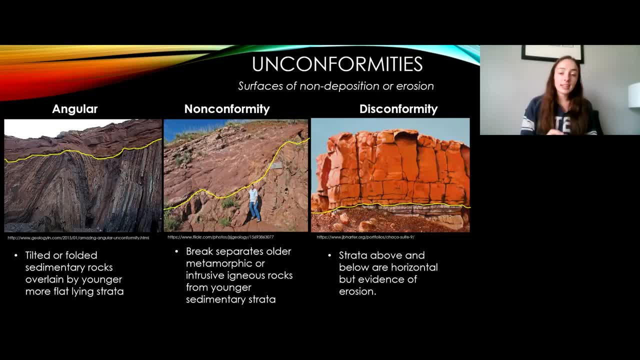 it's harder to tell. but basically this is just saying that there's an erosional surface in between two layers of strata. They can be sedimentary, sedimentary- We just have to be able to tell that erosion occurred. so there's no rock type to tell us the answer. There's no angularity to 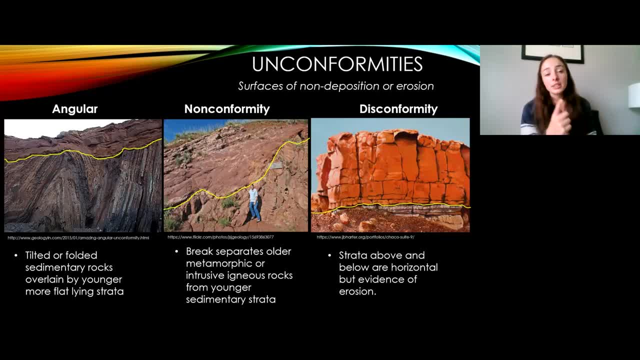 tell us the answer. We just have to be able to tell that erosion occurred. Sometimes we can tell this by rock type, once you go further into detail, If you say, okay, both of these are sedimentary, but let's go into more detail, Is this a limestone? Is this a sandstone? What might? 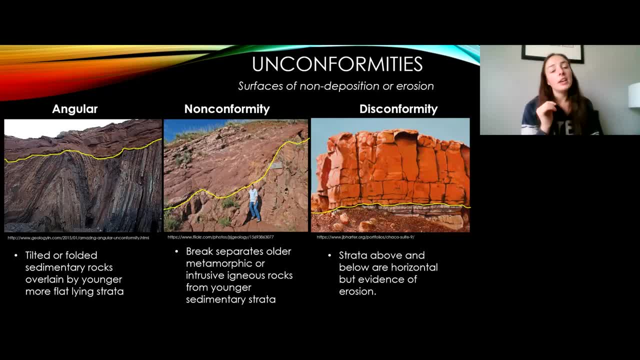 have happened? What's the surface characteristics? So all of these things can help you decide whether that boundary between those two rocks is an erosional surface or not. Those are the three types of unconformities. Moving on, this is an exercise for you guys to think about before I. 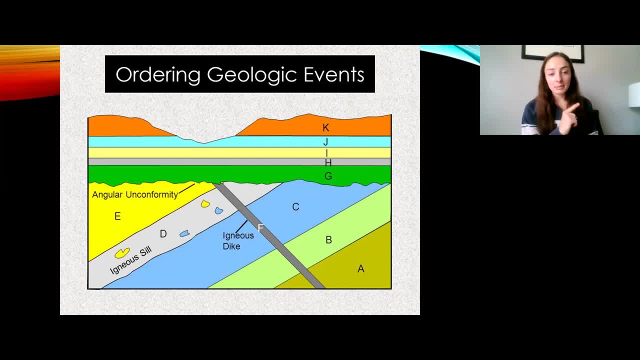 tell you the answer So you can pause the video. but I'm going to ask you a question. you have to think about it. Pause if you need to, because I'm going to say the answer right after I ask the question. What I'm going to ask you first is: what do you think the oldest layer? 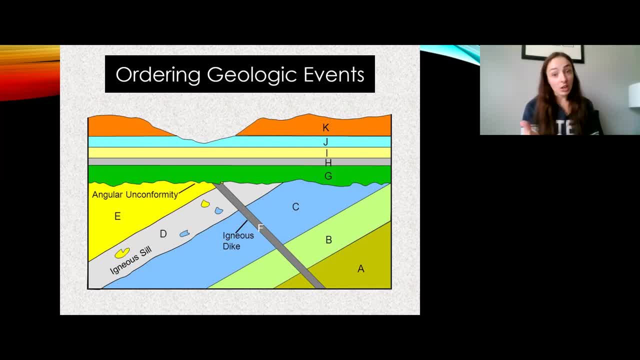 of rock here is. This is basically a cross section of rock layers, and they're just color coded for our ease, And so the oldest rock layer in this sediment should be A, Next the layer that deposited after that was B. The next layer to be deposited was C, Next. this one is tricky. 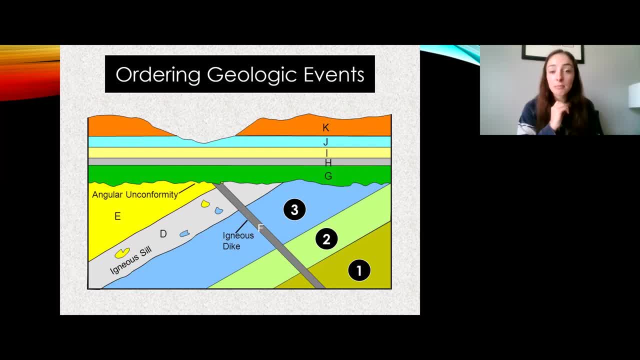 you know, dikes and sills are igneous, so igneous might be younger, So the next one is E. Now, before I move on, let me explain why that this is E. The igneous sill D doesn't come right after layer C. 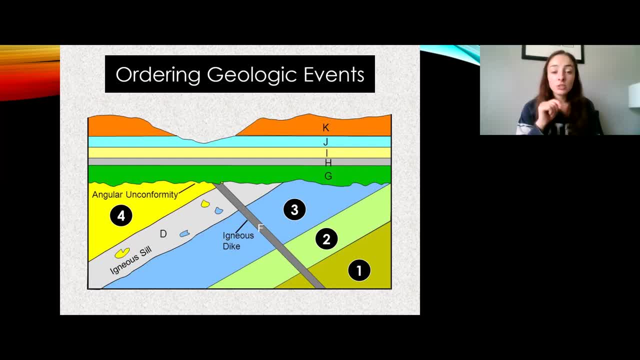 or three. I put the three over the C because you can see that it incorporated material from both layer C and E, which is the blue and the yellow. This indicates that it started intruding after those layers were deposited and it squeezed in between the surface, in between those. 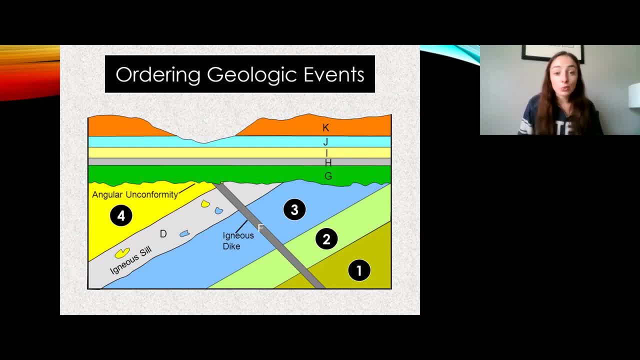 rock layers and it picked up this material because obviously this rock didn't want to move very easily. So if some of it broke off and went into the igneous sill, and that's what we see here, And so that's how we know that this D igneous sill layer is younger, So that's the 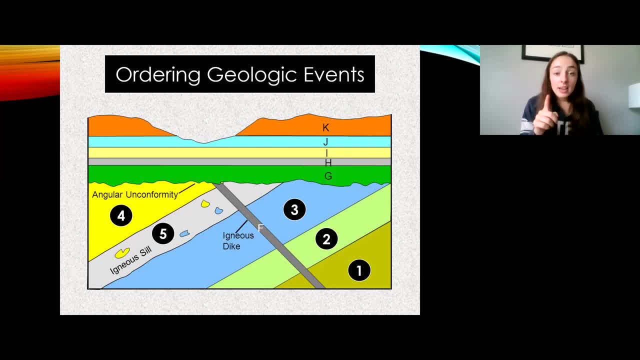 next one. that happened after the blue and yellow deposited Next. we know that this F? igneous dike deposited after all of these angled layers here because it cuts across all of them. We can see it with our eye and we know that this F? igneous dike is cut off by G, meaning that we had 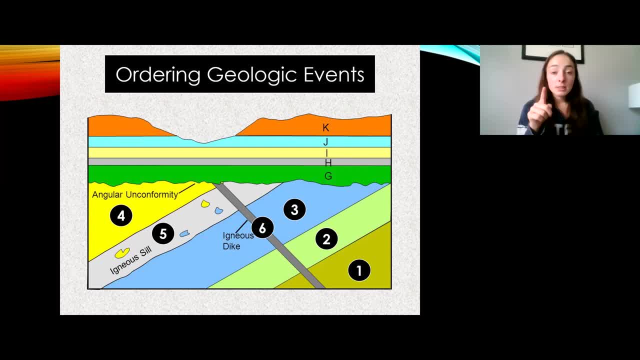 the one, two, three, four, five and igneous dike six, deposit and then erode away. because we can see clearly something folded the layers and then the sill came in and then the dike came in and then there was erosion to take off the top of that fold. 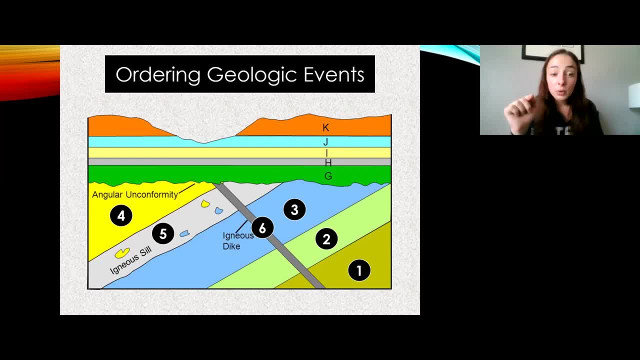 Now they're just angled layers and that's an angular unconformity that is already labeled there for you. that designates the bottom of layer G and that is our next layer, that deposited After G. it gets pretty simple. You have H, I, J, K, So then you have one more. 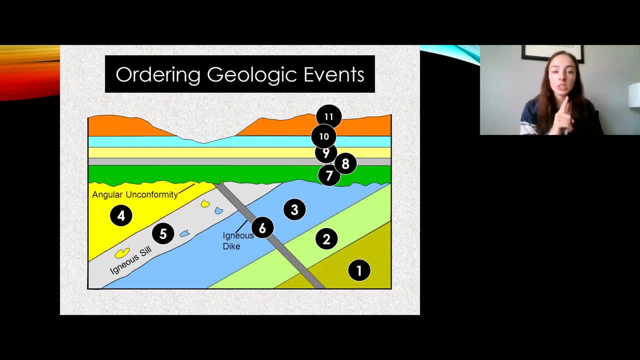 12. Obviously, there's some more layers, but this is ordering geologic events, so we also have to think about events that aren't necessarily rock depositions. So the last event is 12, erosion, and this is important to note, that you're ordering geologic events, not just rock. 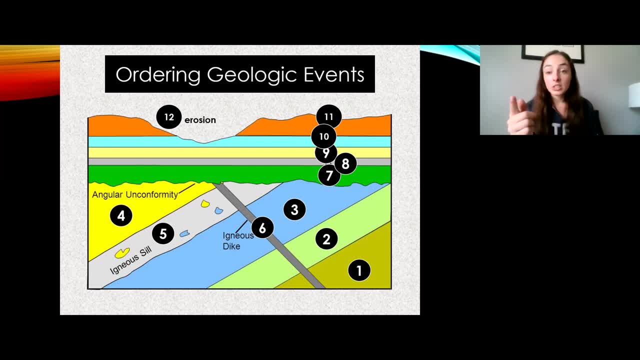 layers, geologic events. so like the unconformity. Actually you should have ordered that as well, meaning I should have, but I didn't, I forgot. but basically that might have been seven and then G would have been eight, so there shouldn't necessarily be 13 events. I messed up. 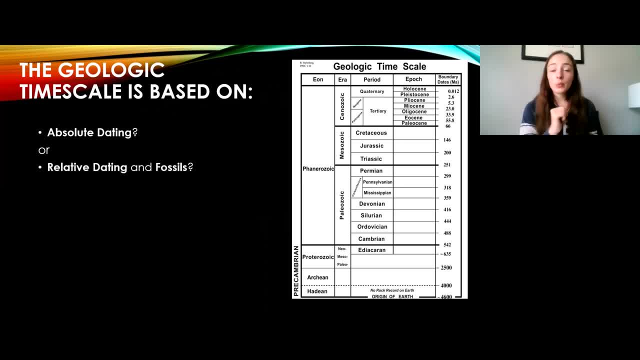 but you get where I'm going. Next, we're going to discuss what is the geologic timescale based on. We see that we have really specific, specific numbers here, but those only came after the timescale was really in place. We built the timescale on relative dating and fossils. We only used absolute dating later, when 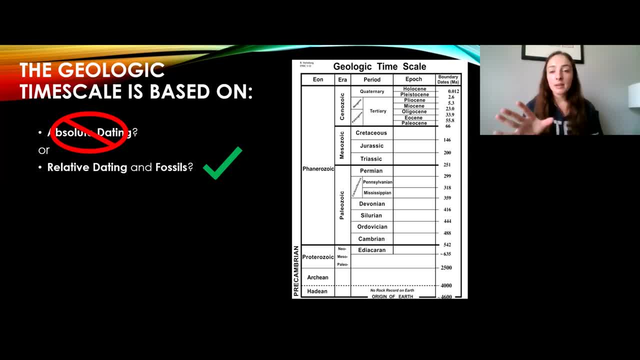 we already had the designated categories of time all figured out and then we came in and absolutely dated a lot of the rock layers that define certain boundaries of time. That's how we came up with the more specific numbers, but originally we did build a timescale based off of relative dating and 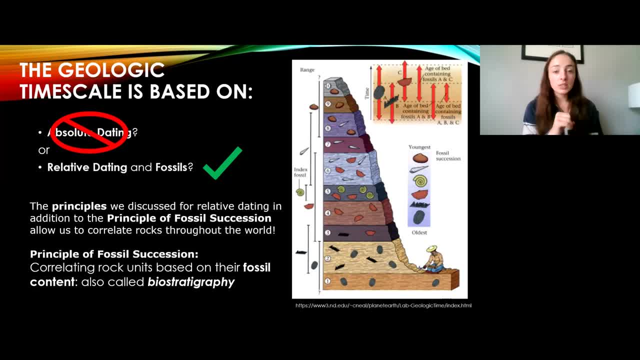 fossils and when you're dating things relatively with fossils. it's called biostratigraphy, and so this is the principle of fossil succession, a principle we didn't talk about earlier because it's so different. I wanted a whole slide for it by itself, but basically, this principle is used. 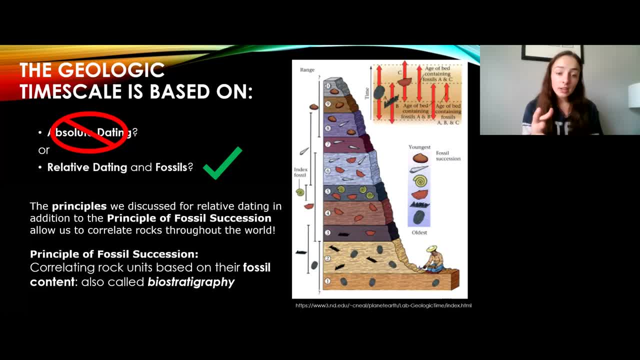 in biostratigraphy, where you date the strata based on biology or the fossil content. so it makes perfect sense. it's called biostratigraphy and what you can see here in this strat column, this is called a stratigraphic column, by the way.